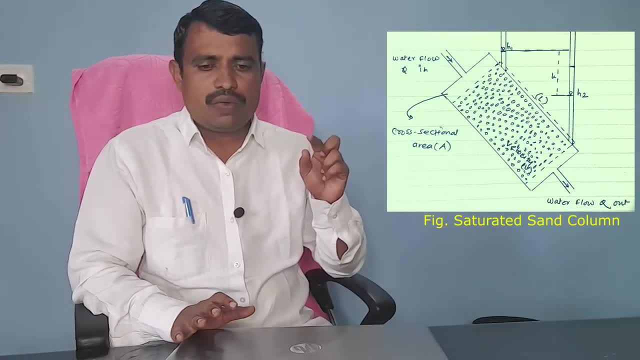 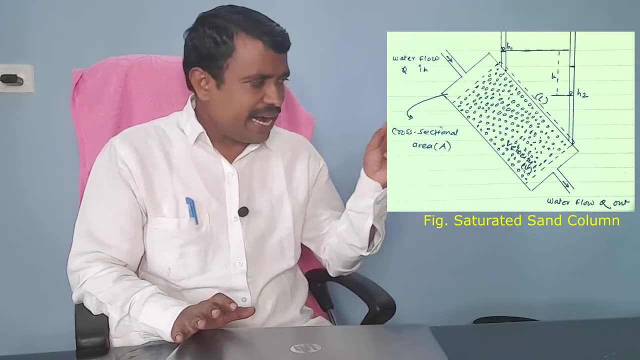 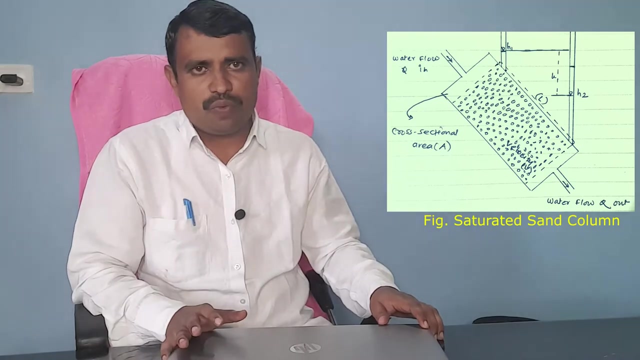 You see, at the two ends, from the upper end there you can see that the water flow quad as Q from where water is entering into that particular sand column, And at the bottom you see there is again second Q, that is the capital Q, that is quad as water flow and from where water is out, pour out from that particular sand column. 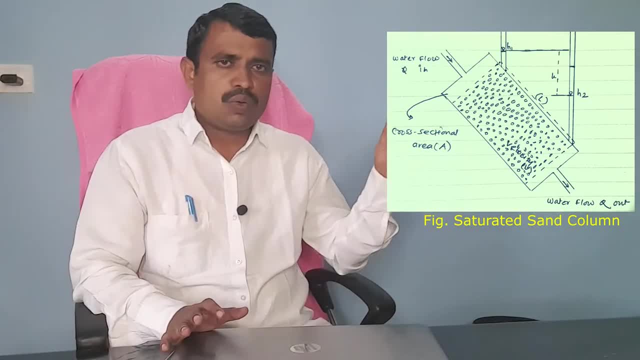 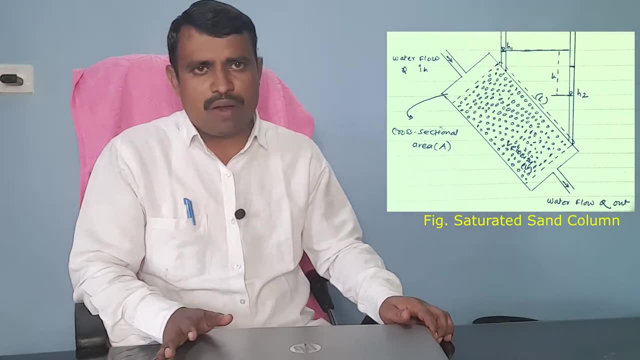 When water is entering into the particular sand column to the end part, or from where water is released, or out from that particular sand column by velocity quad as V. You see in diagram how the velocity you can see moving velocity from one place to another place. 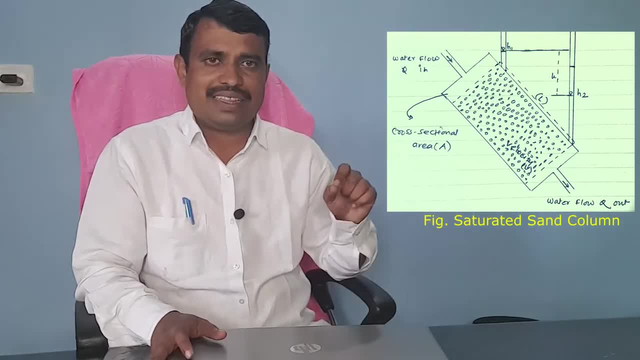 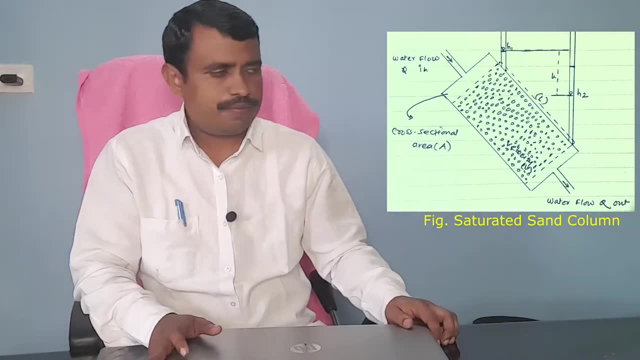 And that column saturated sand column having a particular length called as capital L. You see, at the top there is a length you can see in capital L letter. Other two things are there. One thing is that you can see the what is the cross sectional area. 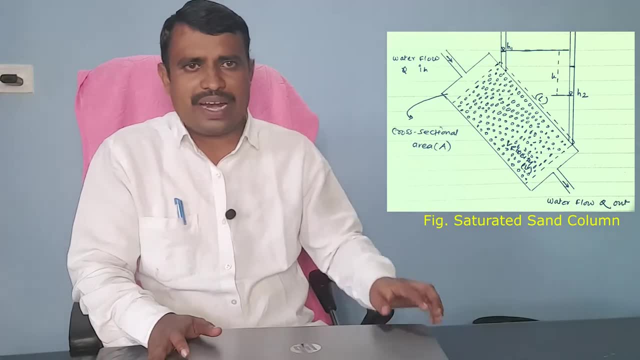 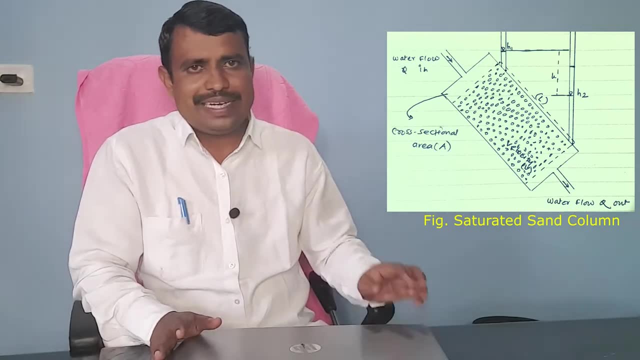 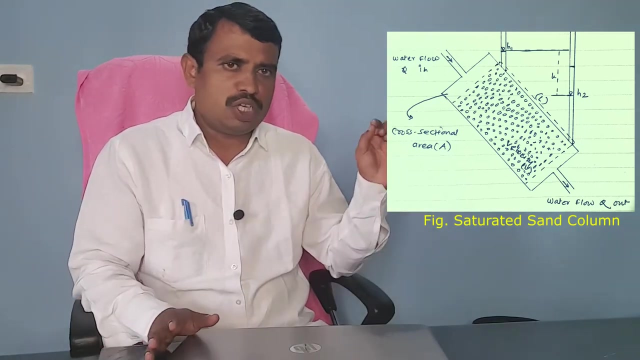 of that particular sand column. So that is denoted by letter A. There are two heads, that is, the H1 and S2.. The difference between H1 and S2, it is nothing but the small h, Because H1 is the top head point and S2 is the lowest end point of that particular sand column. 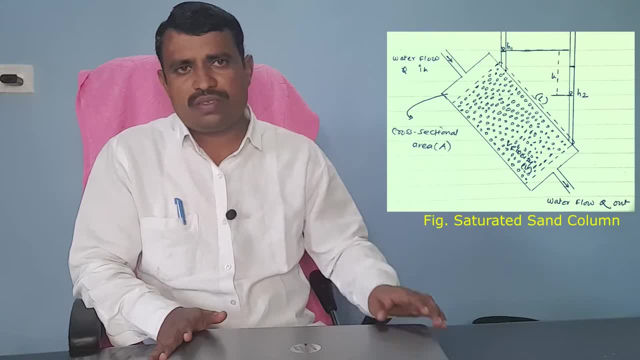 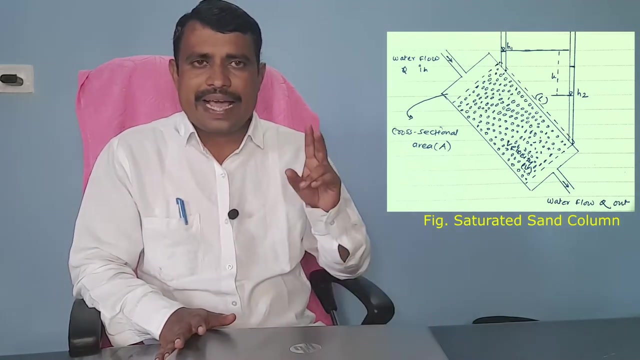 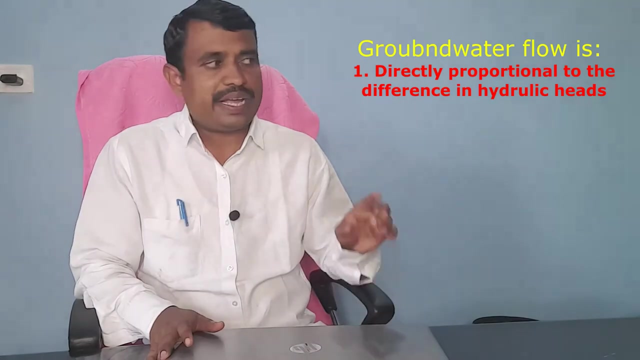 According to the Darcy, when water is flowing through this saturated column, he told two important things regarding the ground water. So when ground water is flowing through the porous medium, or we can say that aquifer, it has two things. When water is flowing through that particular porous medium, it is directly proportional to the head difference. 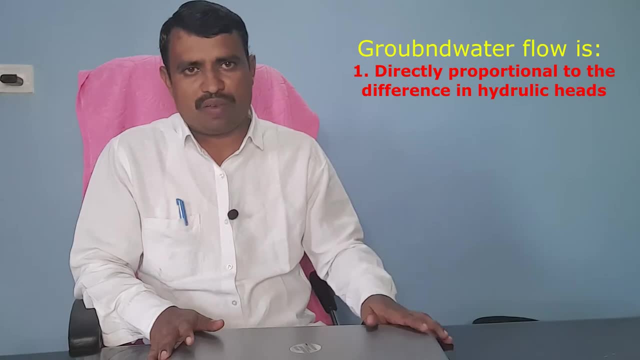 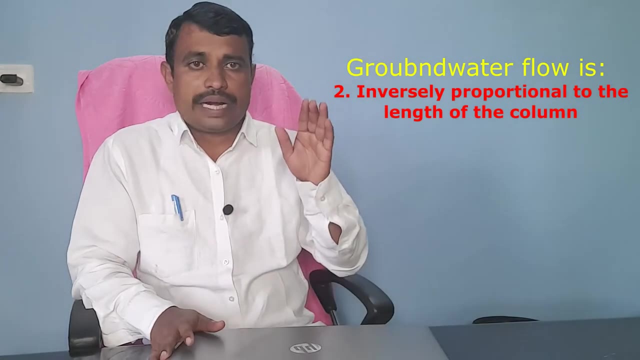 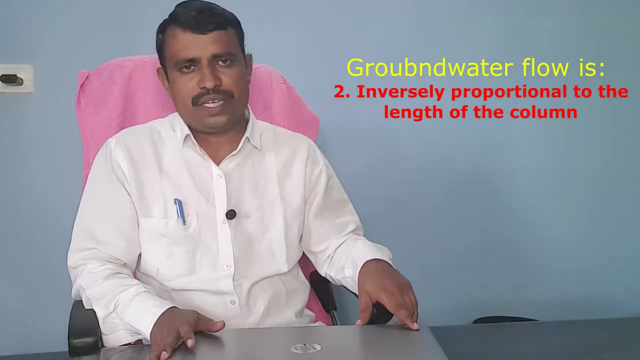 between the two points of the at the end of the column. This is the first statement he did. Second statement Darcy did, that is, the rate of flow of groundwater is inversely proportional to the length of the column. It means that if the length of column is more, water velocity decreases. 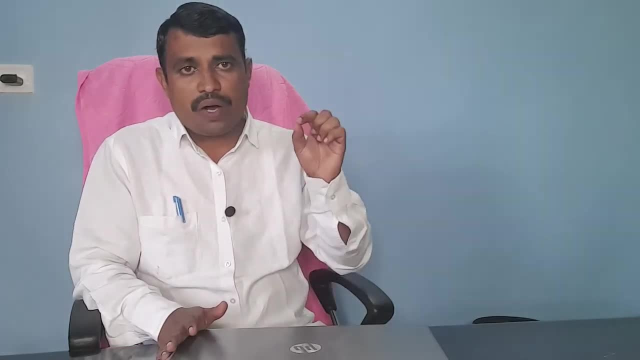 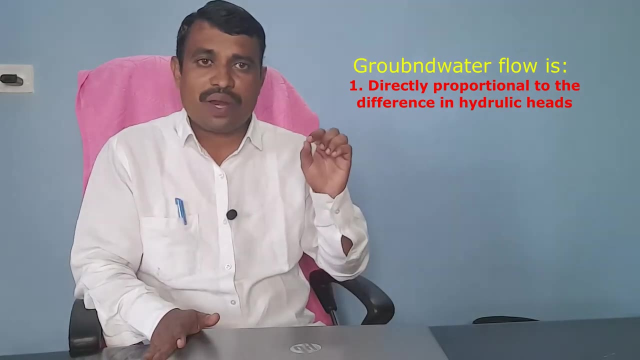 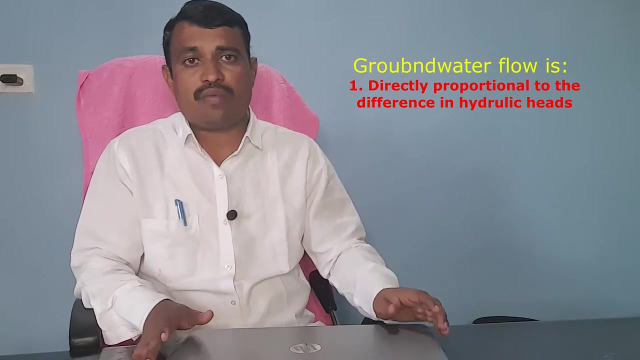 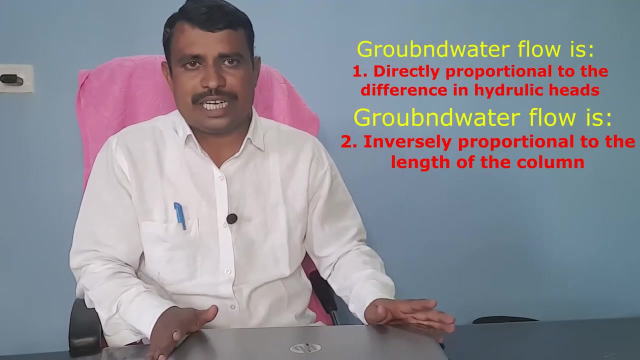 This is the inversely proportional and according to the directly proportional, that is the head difference. if head difference is more, automatically the velocity of water is also more. If head difference is less, the automatically the velocity of water which is flowing through the ground automatically decreases. These two statements we can mathematically, it can be, write it as you can see. 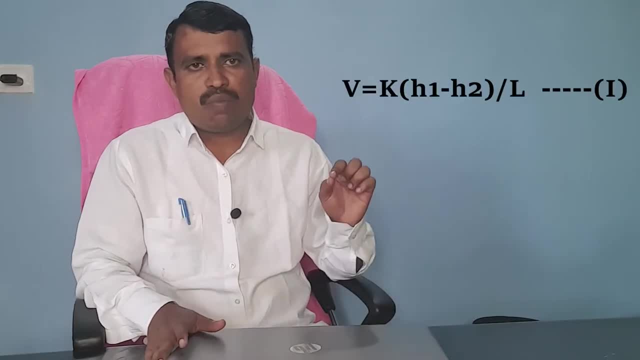 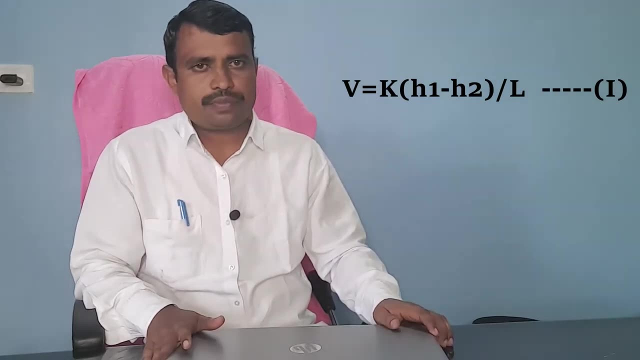 it is equal to k into h1 minus h2 divided by l. So this is the equation we can write in mathematically. So in this equation you can see where phi is nothing but the flux velocity, or it is also called as specific discharge. Then in that equation you can see here. other thing is that that is the 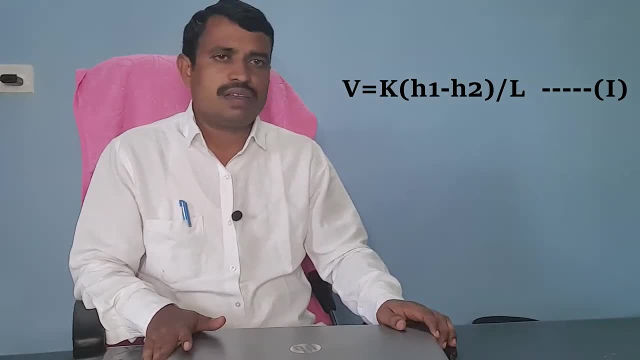 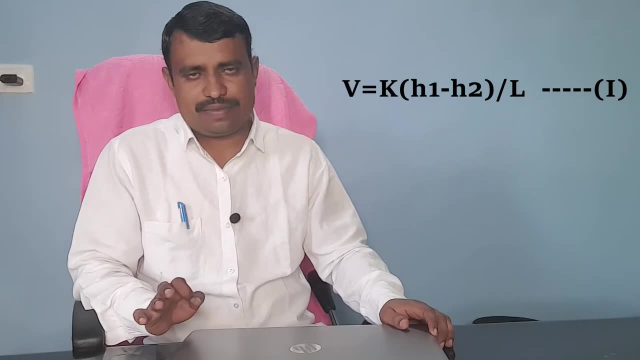 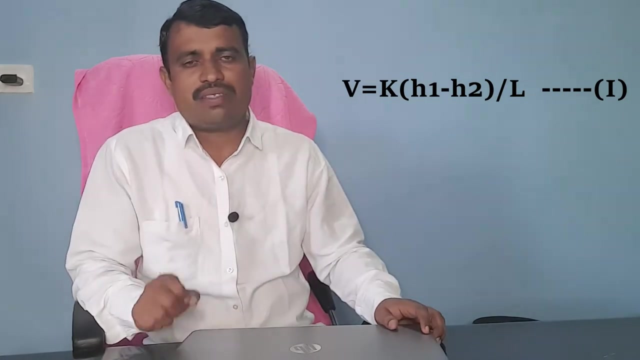 k. k is the constant called as hydraulic conductivity, And h1 minus s2. that is the difference in hydraulic heads. And one more thing in that equation you can see, that is the l. l is nothing but the length of the particular column, or you can. 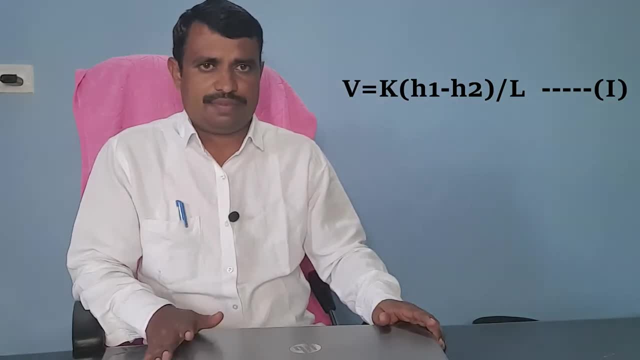 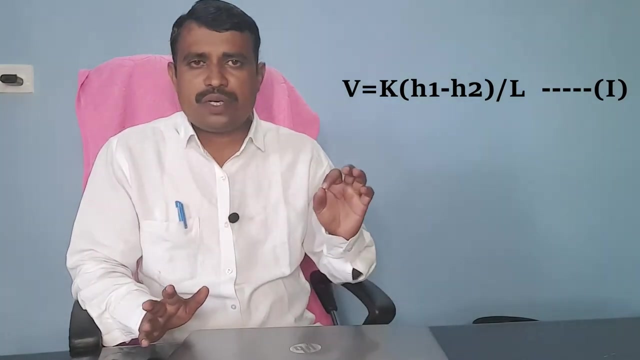 say that this is the length of particular aquifer. So this is the equation: phi is equal to k into h1 minus s2 divided by l. This is the first equation according to the Darcy's law. But when we see this, the difference between hydraulic head and the length of the column, these two things we can write. 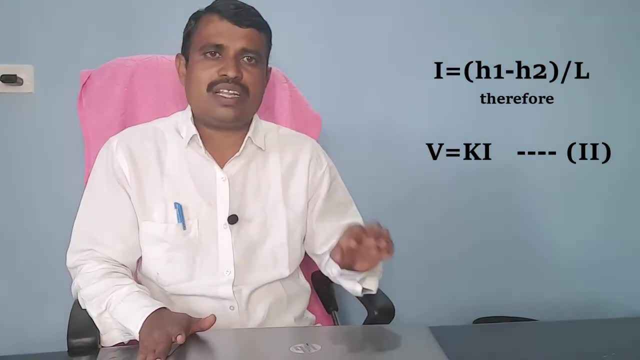 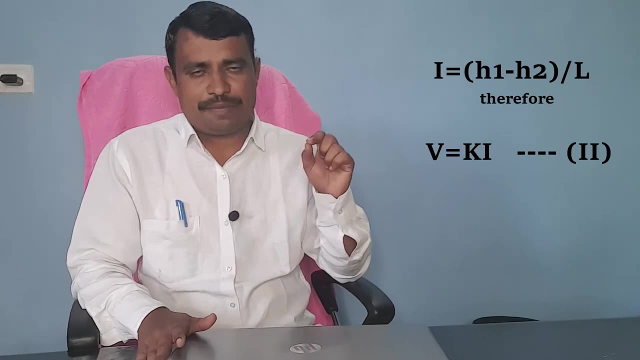 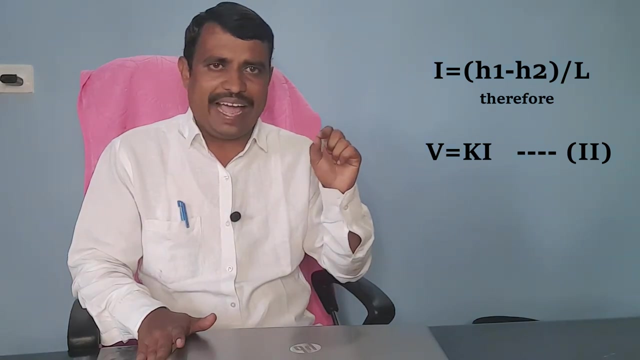 it has by letter. i. i is nothing but the hydraulic gradient. So therefore the second equation becomes, that is, the phi is equal to k into i, So h1 minus s2 divided by l. in place of that particular equation we can write i. So therefore phi is equal to k into i. So this is the second equation. 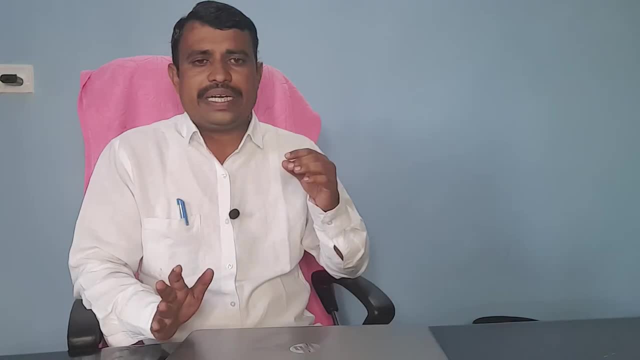 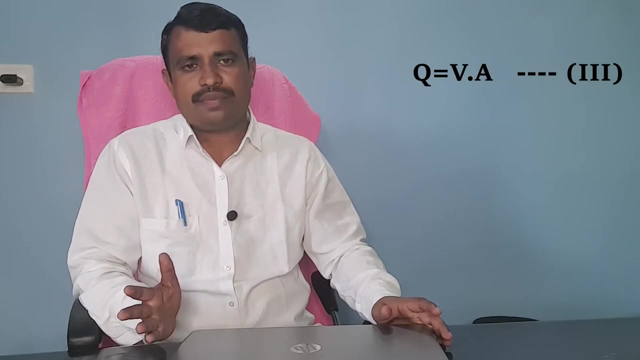 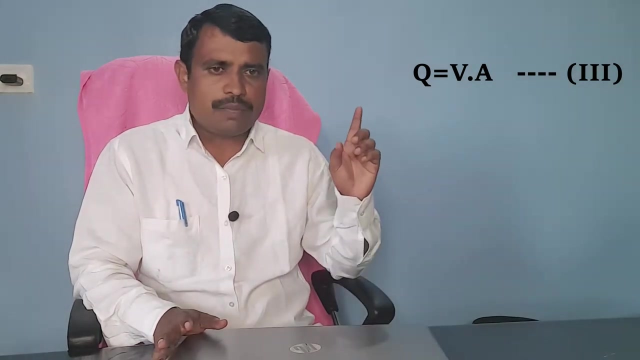 according to the Darcy's law. But it is known that in pipe flow condition, which is analogous to the flow of a porous medium, the discharge q is given by relationship, that is a. q is equal to phi into a. In that particular equation you see where phi is the nothing but the velocity of specific.